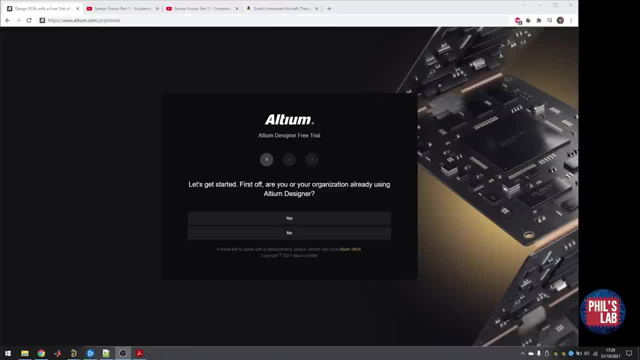 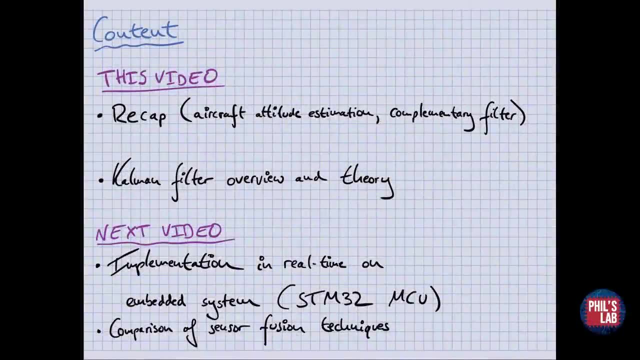 Altium Designer is the main piece of software I use for PCB design, both at home and at home. I'll be showing more of Altium Designer's features in future videos on hardware design, so stay tuned. In this video we'll have a quick recap of the content of the previous two videos on sensor. 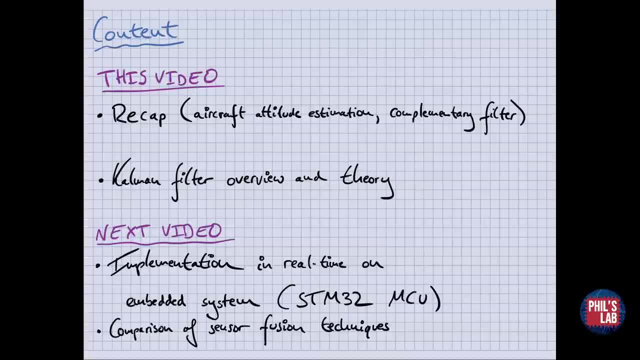 fusion, where we looked at estimating the roll and pitch angles of an aircraft by using a complementary filter. Then we'll go over the Kalman filter, which is a much more effective and configurable way of combining dynamic models with various sensors. Since the Kalman filter is quite involved, I have split the topic into two videos. 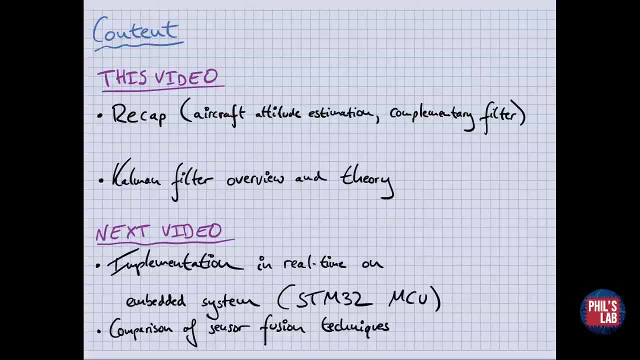 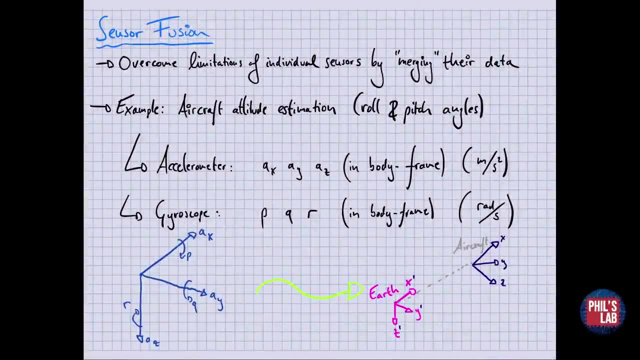 The next video will cover an actual real-time implementation of the Kalman filter on an embedded system. We'll be looking at coding the Kalman filter in C for an STM32 microcontroller and look at some practical implementation considerations. Sensor fusion helps us overcome limitations of using individual sensors by merging data of 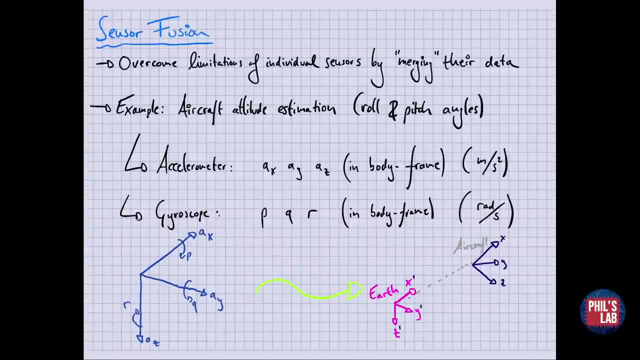 multiple different sensors. For full details, please see my previous videos linked in the description below. We looked at a practical example, that of aircraft attitude estimation. We looked at a practical example, that of aircraft attitude estimation. In particular, we were interested in estimating roll and pitch angles. We have two sensors available. 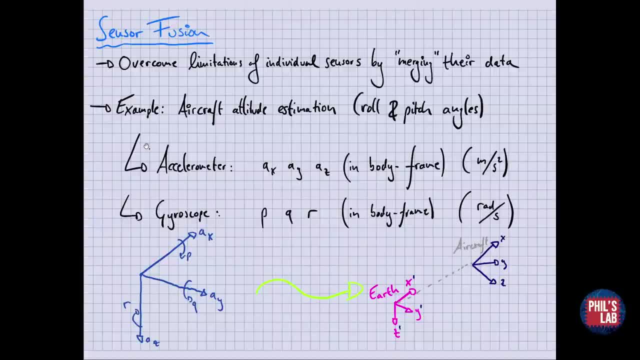 in our example, An accelerometer which measures accelerations in the aircraft's body frame in meters per second squared. We also have a gyroscope which measures rotational rates in the aircraft's body frame in radians per second. Keep in mind that we would like to know the roll. 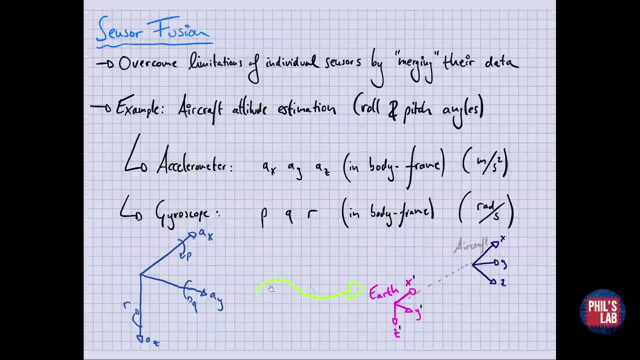 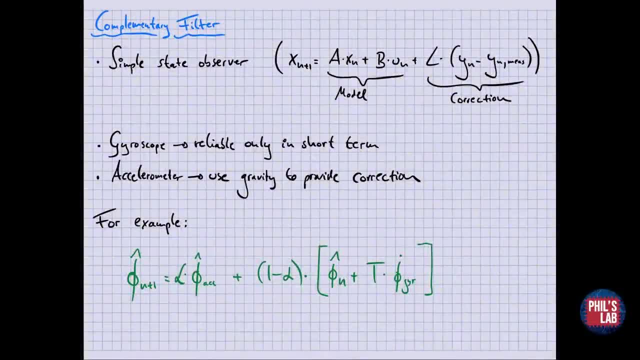 and pitch angles that the aircraft makes with a fixed reference frame. Let's assume the earth's surface is a fixed reference frame. for simplicity, In the previous video we saw that the complementary filter was a very simple but passable sensor fusion algorithm. Essentially it is a simple. 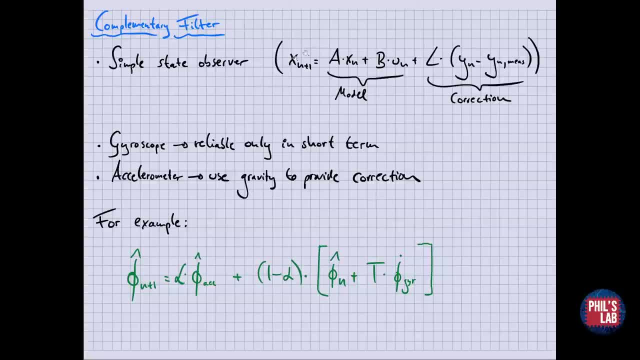 state observer, where we have a dynamic model which updates our state estimate and a correction term which aids against drift. We saw that gyroscopes are only really helpful over shorter periods due to the phenomenon of gyro drift. On the other hand, accelerometers are useful only for 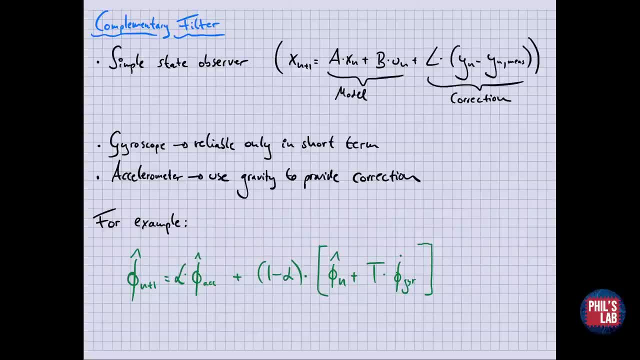 long-term corrections. The complementary filter, however, is incredibly computationally effective, as is seen in the equation over here. The accelerometer estimate over here is combined with the integral of the gyro readings to get an update of the roll angle. Take a note of the constant alpha. 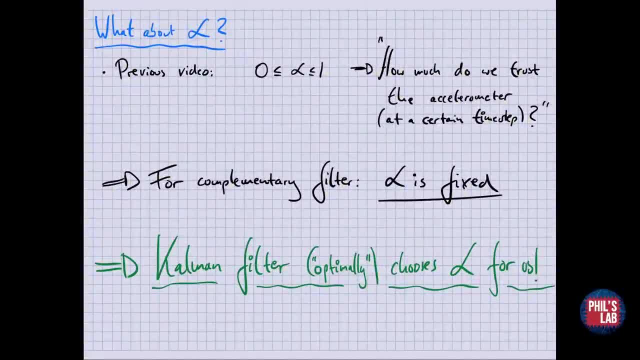 From the previous video. alpha is a constant between 0 and 1.. A rough explanation of alpha is: how much do we trust the accelerometer measurements at a certain time step? Note that for the complementary filter, alpha is fixed. However, as we'll soon see, 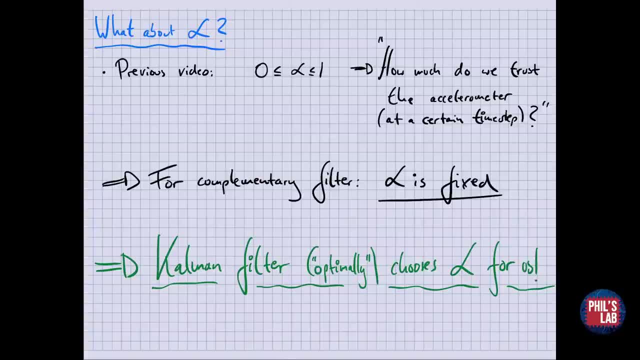 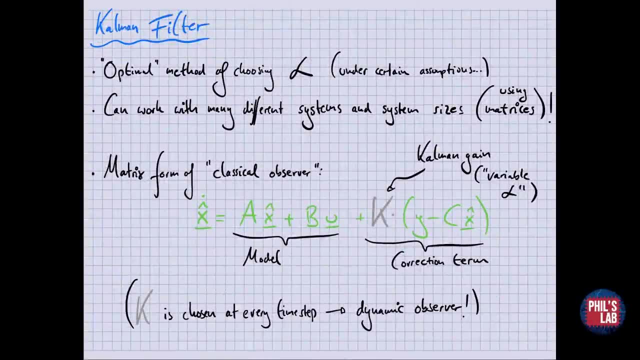 the Kalman filter optimally chooses alpha for us. However, we have to be careful of what we mean by optimally. Under certain conditions and assumptions, the Kalman filter is actually the optimal way of choosing alpha. In addition, the Kalman filter 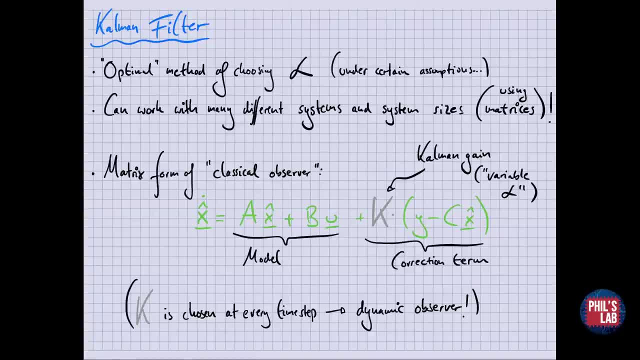 doesn't have to be scalar, which means it can work with many different systems and system sizes by using matrices. We start our analysis of the Kalman filter by looking at the matrix form of a classical observer. Note that the hat denotes a state estimate, a bar underneath a variable. 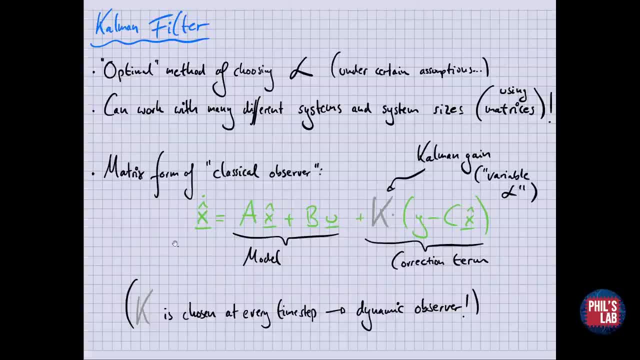 letter denotes a vector and an uppercase letter denotes matrices. The observer model consists of a dynamic model given by ax plus bu and a correction term which is some coefficient times a measured term minus a modelled estimate, As opposed to the complementary filter. 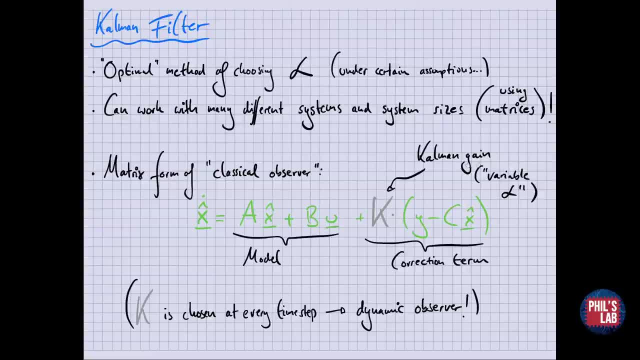 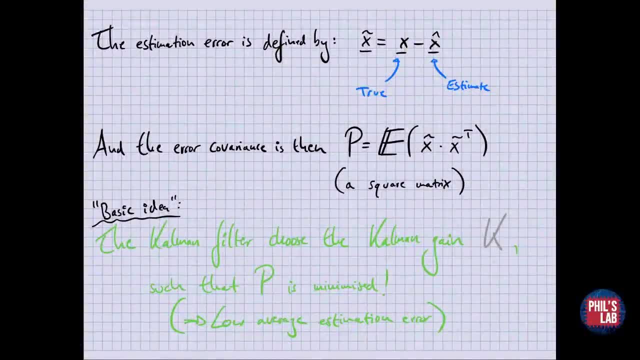 the alpha term is now replaced by a matrix k named the Kalman gain. K is chosen at every time step and thus makes this observer dynamic. We can define an estimation error by subtracting the true state minus our state estimate. Essentially, the larger the state. 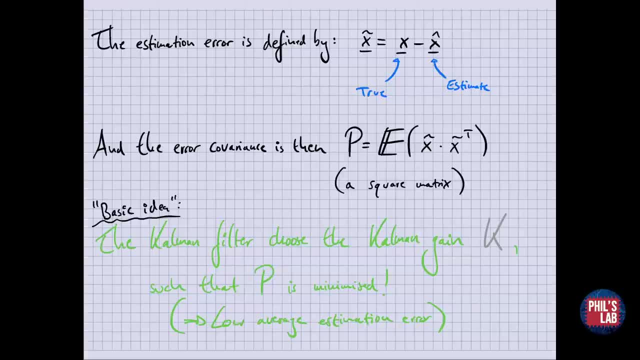 the worse our estimate is and the further our estimate is away from the true state. If we multiply the estimation error by its transpose, in essence some sort of squaring of the estimation error. then take the expectation, in other words the average. 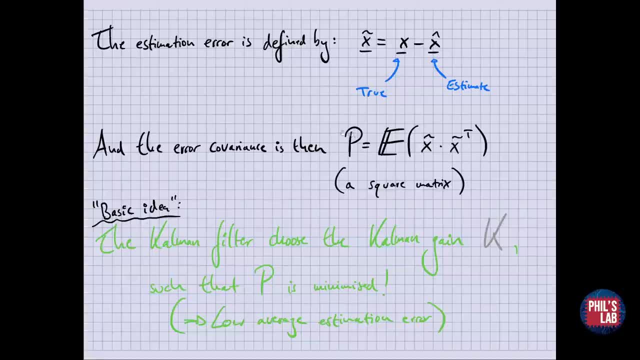 then we get a matrix called the error covariance matrix, p. This matrix is square. The basic idea of the Kalman filter and how it is derived is that the Kalman filter chooses the gain k, such that p is minimised If we have a small magnitude of p. 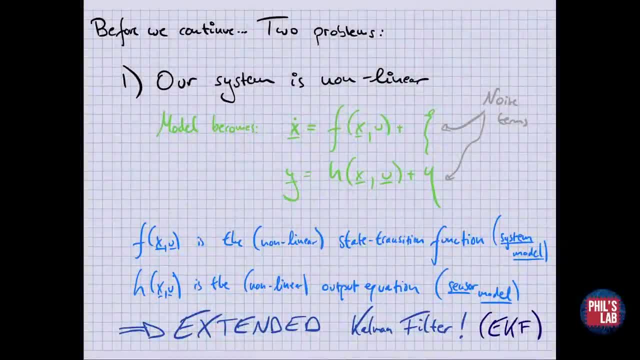 then we can assume a low average estimation error. Before we continue with our discussion on the Kalman filter, we need to fix two problems. Firstly, our system is typically non-linear. We move from our linear model, which is maybe x equals ax plus bu, to a non-linear description by the means of a non-linear state transition. 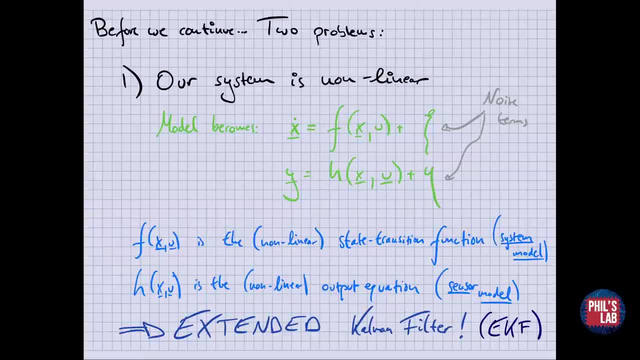 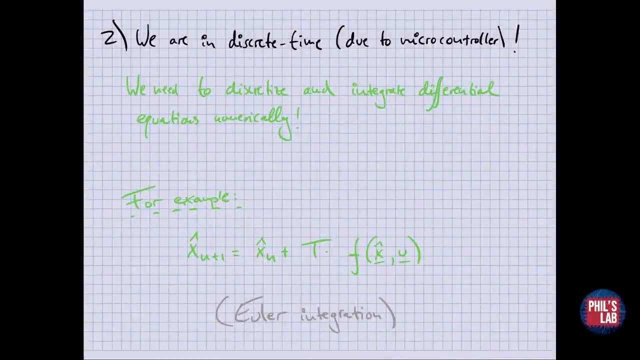 function called f, which is the system model. We also have a non-linear sensor model given by the function h. The non-linear version of the Kalman filter is then called the extended Kalman filter, or EKF for short. Secondly, we are in discrete time, since we will be implementing this filter on a digital 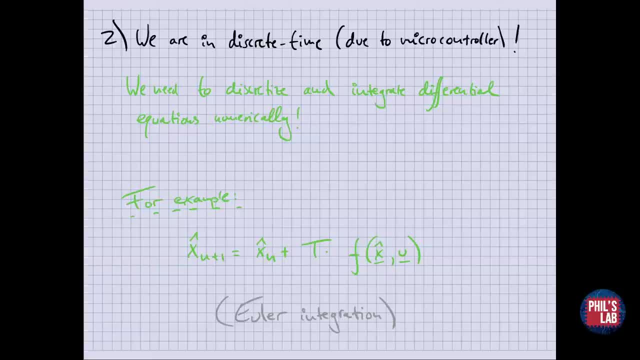 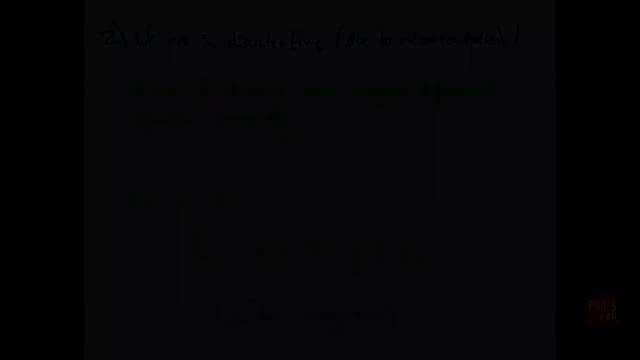 discrete microcontroller. Thus, we need to discretise our models and integrate the differential equations numerically. One way of doing this is via Euler integration, for example. However, we will not be covering the derivation of the extended Kalman filter in this video. 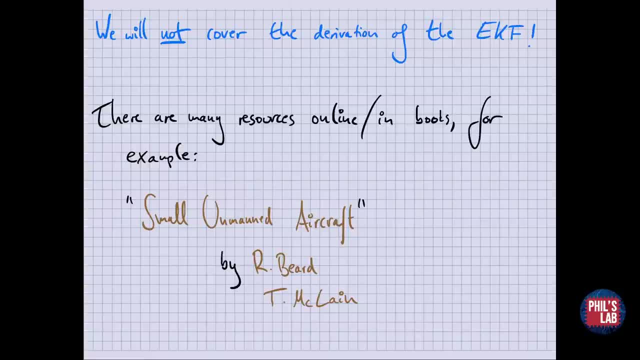 There are plenty of resources, both online and in textbooks, that describe this. One of my favourite examples, and the whole book in general, is Small Unmanned Aircraft by Beard and McLean, and this is the book I'm speaking of. Let's get to the actual EKF algorithm. 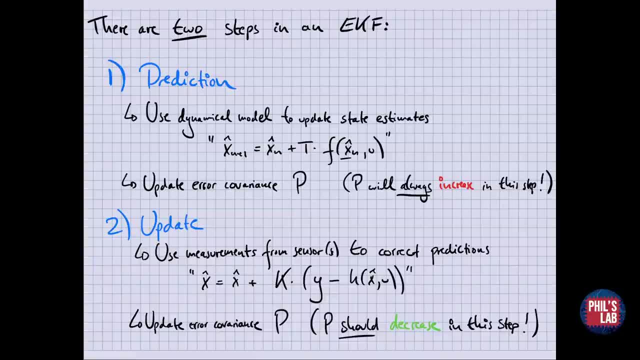 For all EKFs. there are two steps. Let's go over them broadly here and then in much more detail in the remainder of this video. Firstly, the prediction step. We use a dynamical model to update our state estimates. In our case, 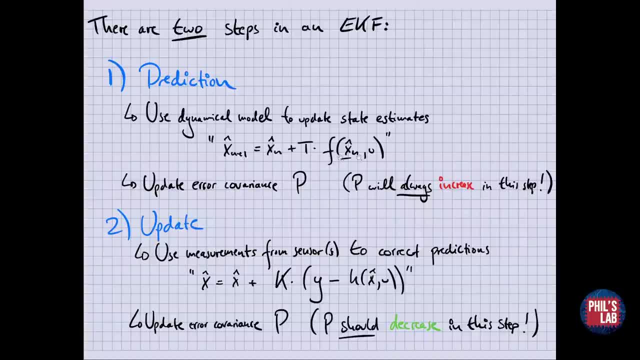 the roll and pitch angles. We do this in discrete time by integrating our state transition function into Euler integration. Remember, our state transition function can be non-linear and is described by f. We'll get to what our state transition function is shortly. 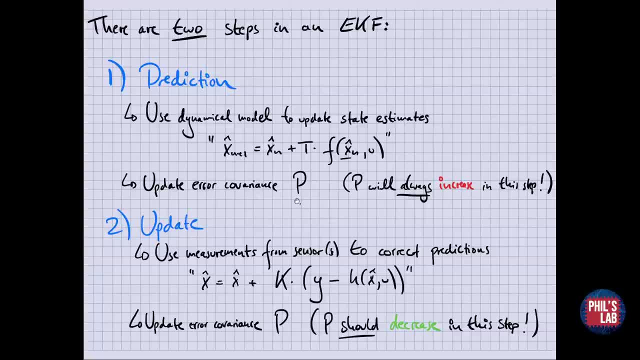 After that we need to update our error covariance matrix P, and remember: P gives us an indication of how well our state estimator, ie the Kalman filter, thinks it's performing. In this step, the magnitude of P will always increase. Thus we are less confident in our 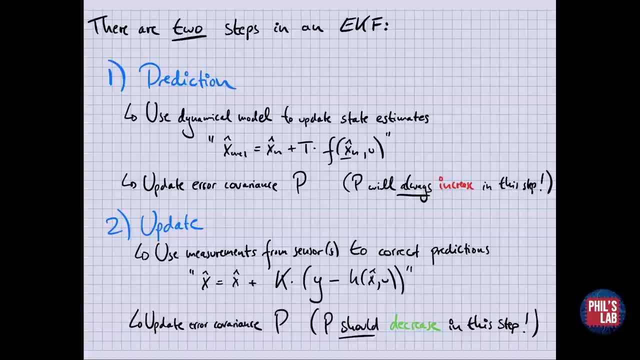 state estimates. The second step is the update step, where we receive measurements from sensors. We'll use these measurements, together with a sensor model, to apply corrections to our predictions. This is where the Kalman gain k comes into play, As with the prediction step. 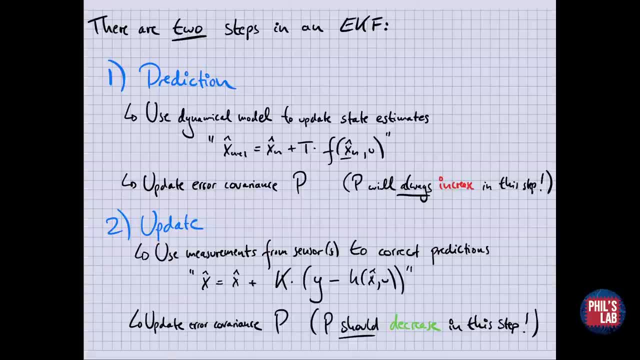 the update step also requires an update of the covariance matrix P. Now, since we are using observations, in other words sensor measurements, our confidence on our state estimates should increase, and thus the magnitude of P should decrease. Now let's go through a practical 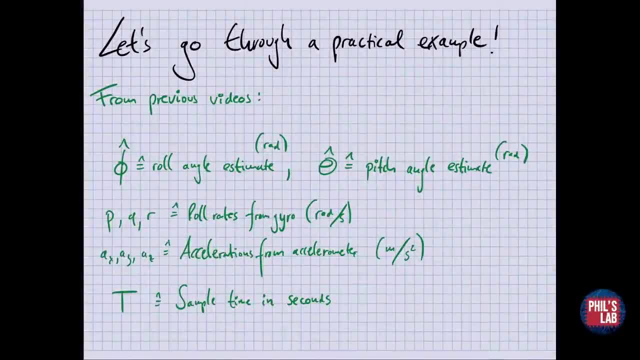 example, that of aircraft attitude estimation. But before let's remind ourselves of some terms that we need to know. Phi and theta denote the roll and pitch angles respectively, and are both in radians. The hat above the Greek letter tells us that this is an estimate. Our sensors provide us with roll. 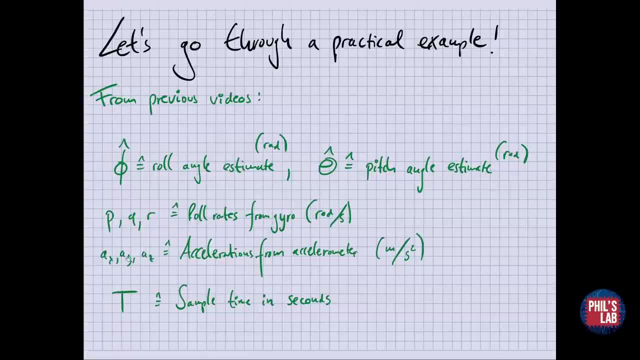 rates P, Q and R in radians per second and accelerations AX, AY and AZ in meters per second, squared along the body axes. We also have a sample time, t, which is in seconds, As we saw. 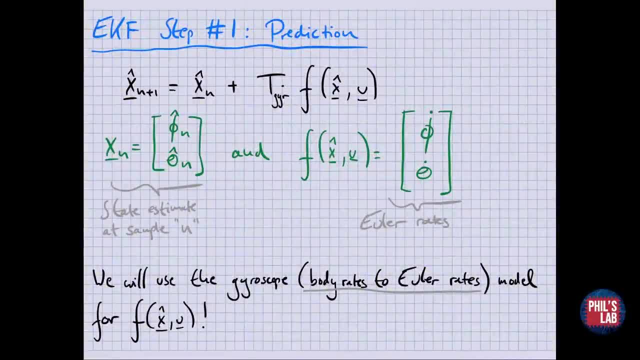 the first step of our EKF is the prediction step. Here we update our state estimate by integrating our non-linear state 2.0. This is the first step of our EKF, which is the prediction step. Here we update our state estimate by integrating our non-linear state 2.0. This is the prediction step. 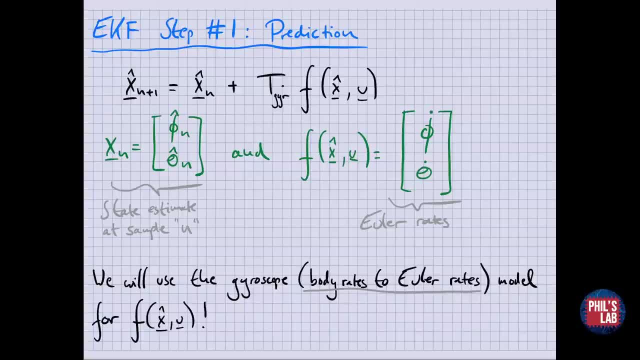 transition function FxU. numerically, In our case, this prediction step is called whenever we have new gyroscope measurements. The state estimate donated by X is a column vector composed of our roll and pitch angle estimates. The state transition function FxU gives us expressions for the rate. 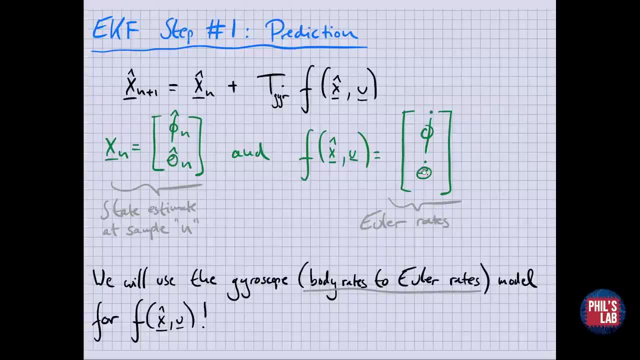 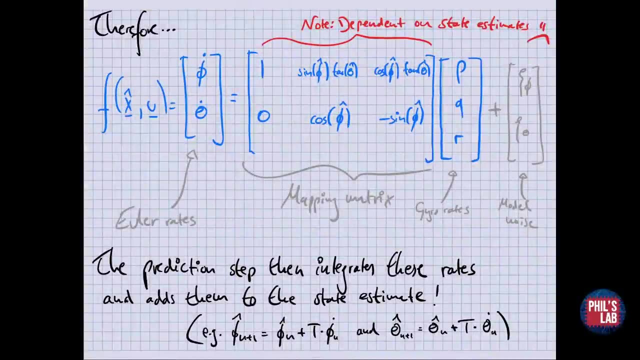 of change of our state estimates, so phi dot and theta dot, In our case the rate of change of roll and pitch angles with respect to time. We will use the gyroscope model which gives the body rates to Euler rates conversion for FxU, which is our state transition function. Therefore our non-linear 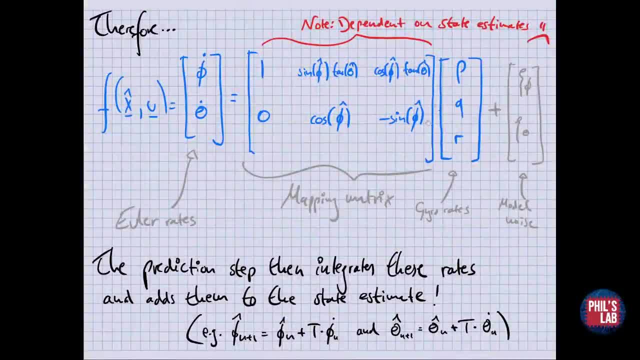 state transition function becomes as shown. The gyro or body rates, PQR are mapped via a matrix to Euler angles, phi, dot and theta dot. Additionally, we have some additive noise due to our model being imperfect and the effect of sensor noise. Also, note that the mapping matrix is dependent on 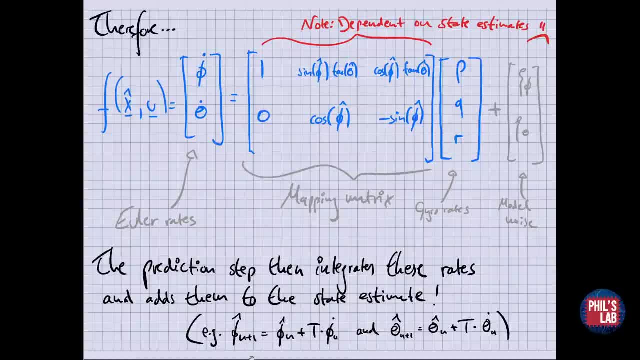 our current state estimates, which isn't great. The prediction step then integrates these Euler rates via Euler integration and adds them to the current state estimate. These are, then, our new state estimates. We can't forget to also update our error covariance matrix P. This is done via the 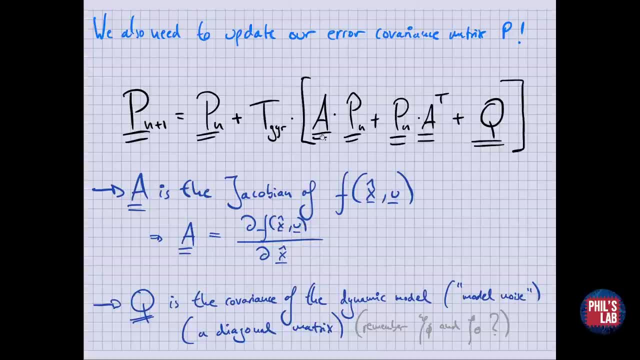 following formula. We can see two new matrices here: A and Q. Now, A is the Jacobian of our state transition function. In other words, its elements are the partial derivatives of the state transition function with respect to the state estimate vector. Now, this is quite a mouthful, but we'll see in the 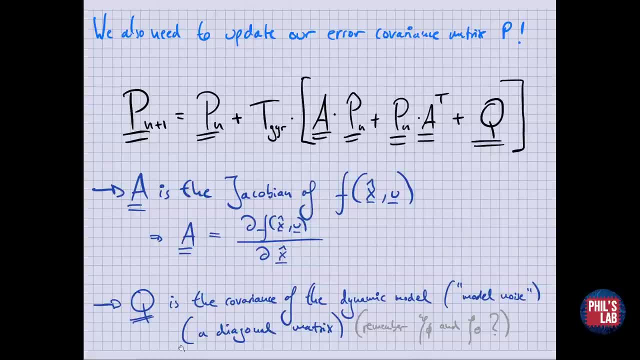 next slide that this is actually quite simple to compute. Q, on the other hand, is the covariance of the dynamic model in most cases a diagonal matrix. We can see it as our model noise. We'll see how we can estimate this in the next video. 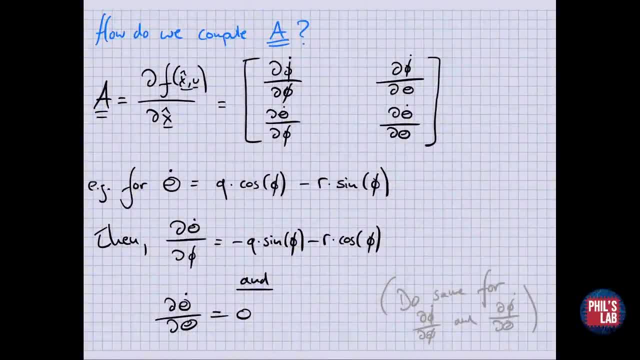 Now the question is: how do we compute the matrix A? As we said before, the elements are the partial derivatives of the state transition function with respect to the elements in our state vector. For example, our state transition function for the pitch angle rate is given here, So theta dot equals. 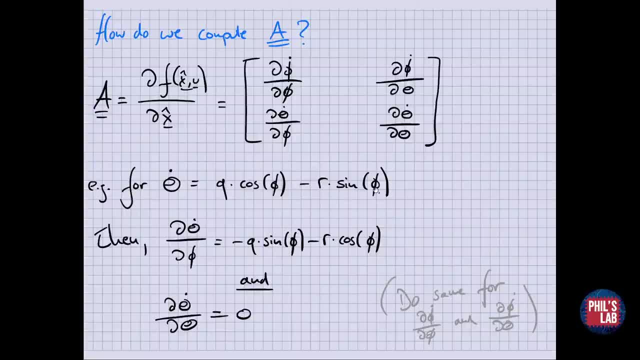 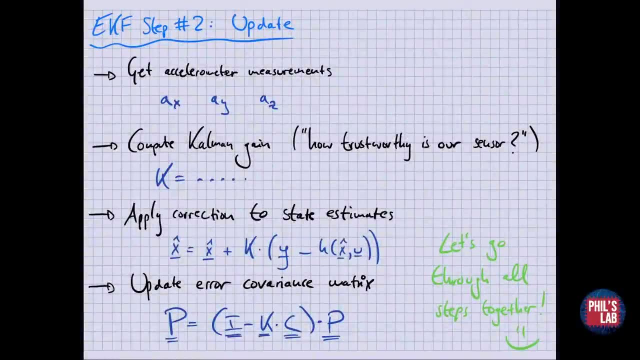 was q times cosine of phi minus r times sine of phi. Then we take our derivative of phi dot with respect to the roll angle as well as with respect to the pitch angle, Then we do the same for the roll angle rate, and that's all there is in a in our case. The second part of the EKF algorithm is: 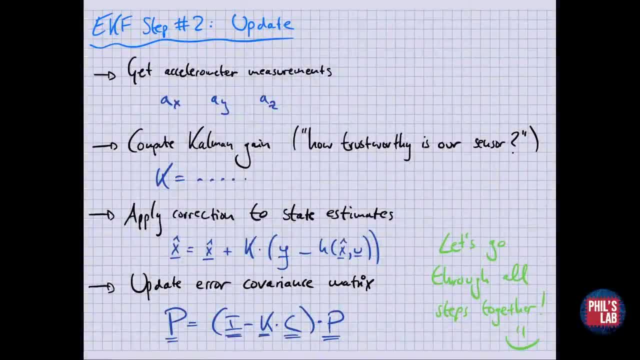 the update step. In our example, this happens whenever we get new accelerometer measurements- AX, AY and AZ. We then need to compute the Kalman gain, which, simply put, tells us how trustworthy our sensor measurements are compared to what our model predictions say. Then we apply this correction. 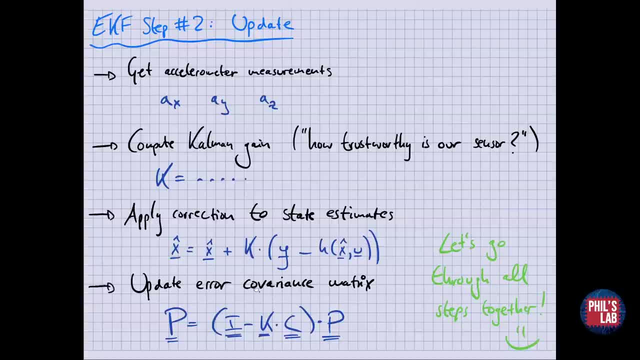 to the state estimates by using a sensor model and the actual observed sensor data. Finally, and as usual, we need to update the error covariance matrix P. Let's go through all of these steps in a bit more detail together now. From previous videos, we described the model of our accelerometer. 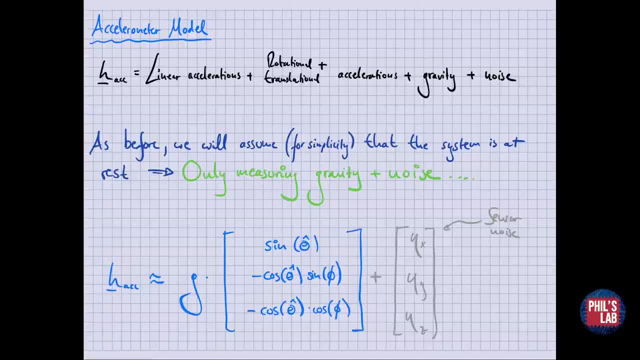 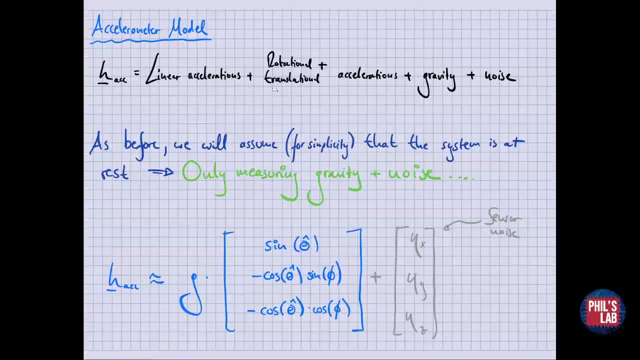 linear accelerations, accelerations due to rotation and translation, gravity, as well as additive noise and possibly a time varying bias. As before, we will assume for simplicity, that the accelerometer is at rest. This lets us eliminate most of the terms, except for accelerations due 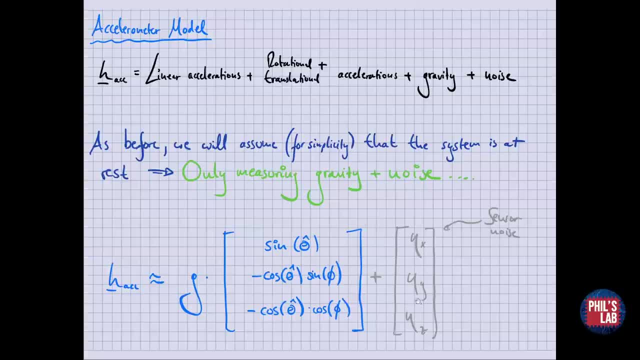 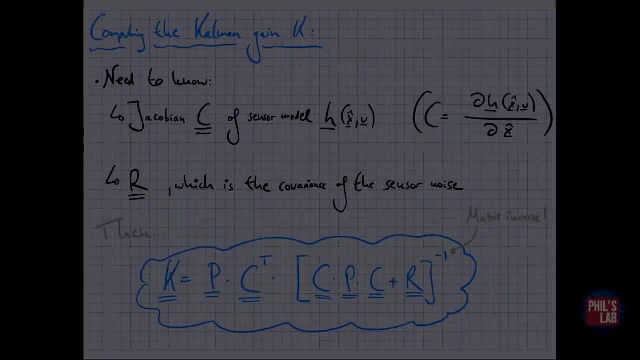 to gravity and the noise terms. Our sensor model denoted by h then becomes this over. here Again, our sensor model is unfortunately dependent on our computer, but we can do that with the current state estimate. The next step is then to compute the Kalman gain k, Remember this was. 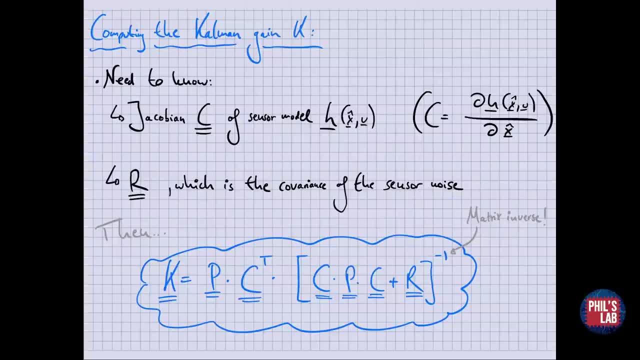 analogous to the complementary filter alpha and is used to correct the prediction step. To compute the Kalman gain, we need to know our sensor model from the previous slide and its Jacobian, which in this case is c. This is very similar to a, which was the Jacobian of the state transition function. 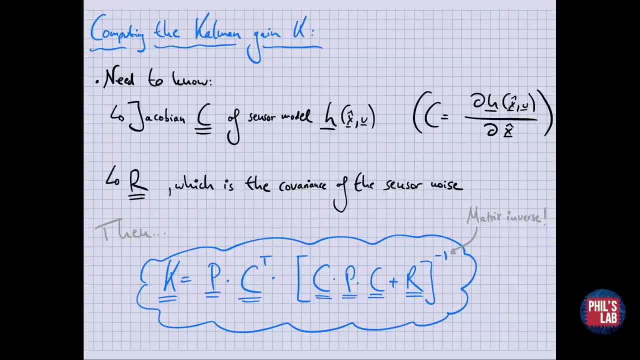 Additionally, we need to know the matrix r, which is the covariance of the sensor noise. In the next video we'll look at how we can estimate that. Then the Kalman gain is given by the following equation, and note that we need to perform several matrix multiplications and a matrix inversion. 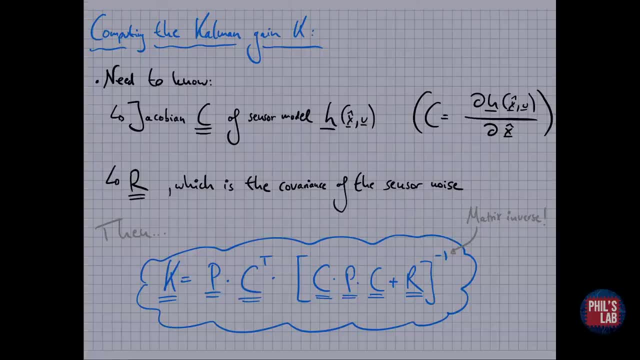 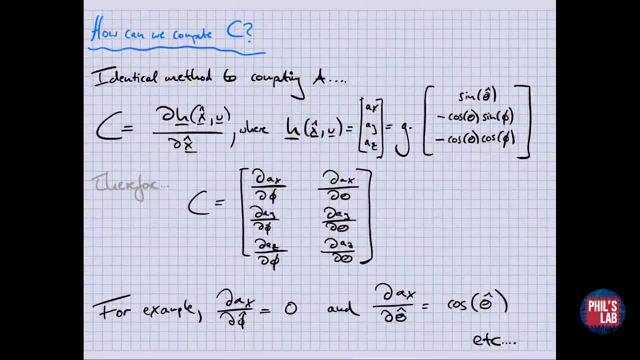 which are quite computationally expensive. but more on that later. As before, computing the Jacobian c is done via an identical method to that of computing the Jacobian a For the matrix c. its elements are simply the partial derivatives of the sensor model h. with respect to the elements. 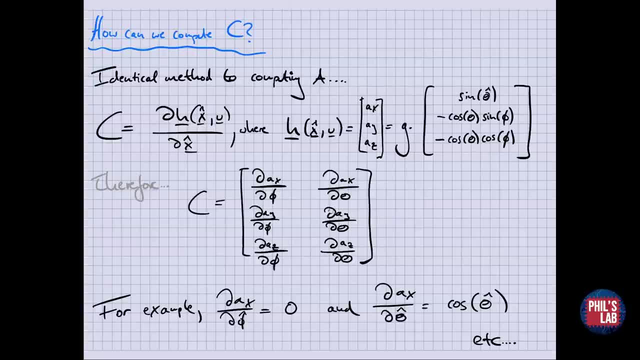 of the state estimate vector. For example, for the first row of c we can compute the elements to be zero and the cosine of our pitch angle estimate. We then do the same procedure for the remaining rows. Once we've computed our Kalman gain k, we 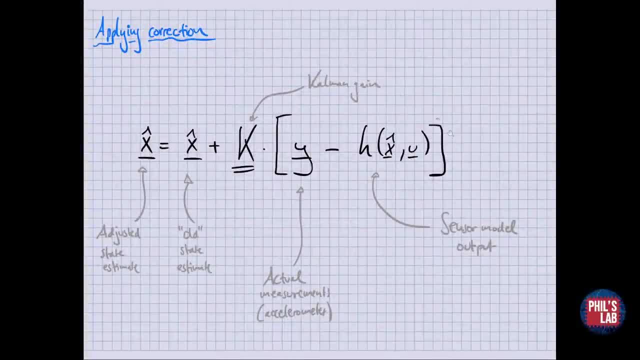 need to use it to apply correction to our state estimate, and this is shown here. We take our actual accelerometer readings, which is given by the letter y, and subtract this from our sensor model outputs, which is denoted by hxu. Our sensor model outputs essentially tell us what we think. 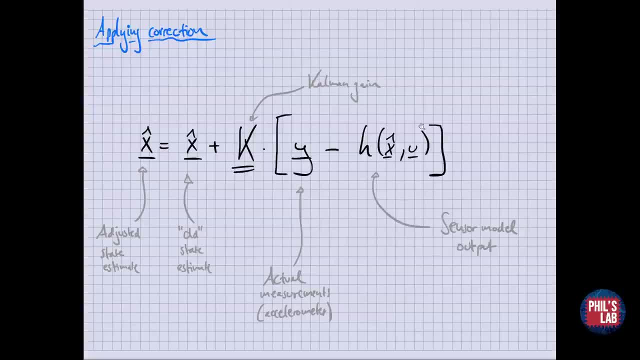 the accelerometer measurements should be Based on our model. this term over here, then multiplied by the Kalman gain, is added to our old state estimates, those acquired by the prediction step. Now it is quite clear to see that if the magnitude of k is close to zero, we prefer or trust the prediction step state estimates. However, if the 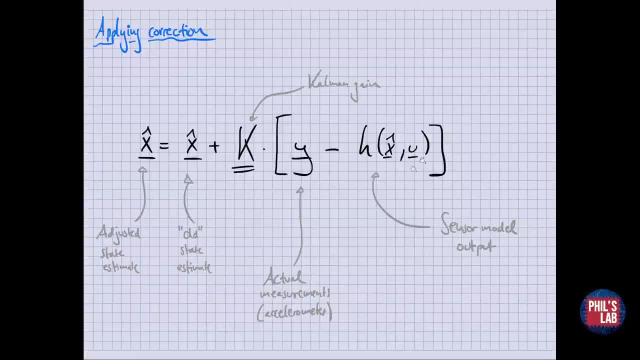 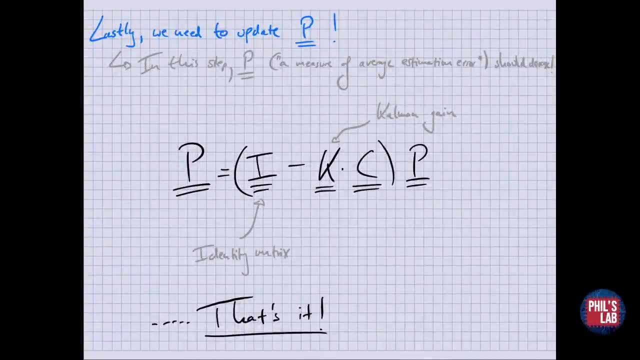 Kalman gain magnitude is larger, we tend to prefer or trust the predictions given by our sensor model. Lastly, and as usual, we need to update the error covariance matrix p. In this step, p which, loosely speaking, is a measure of average estimation, error should decrease. The equation for p is given here and again includes the Kalman gain, k and. 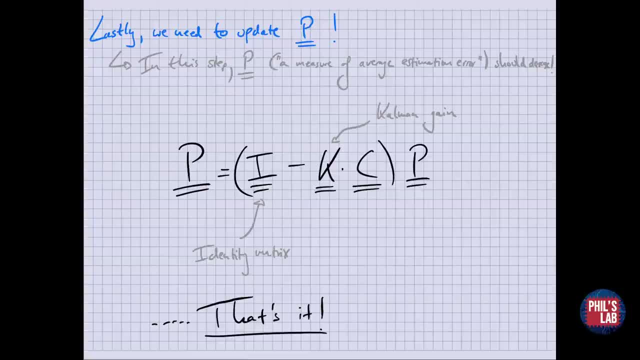 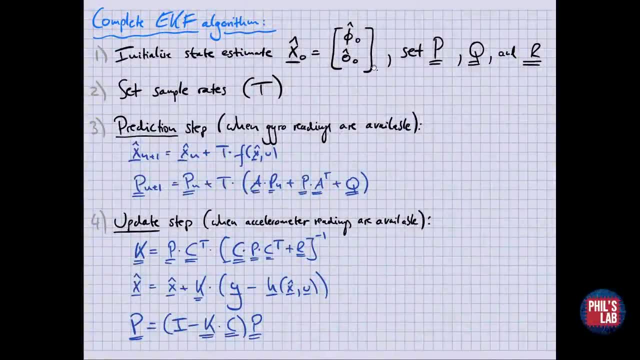 that's pretty much all there is to the extended Kalman filter algorithm. Here's an overview of the complete algorithm. We initialize our state estimate, which in our case is a column vector containing our initial estimate of the roll and pitch angles. We also need to initialize 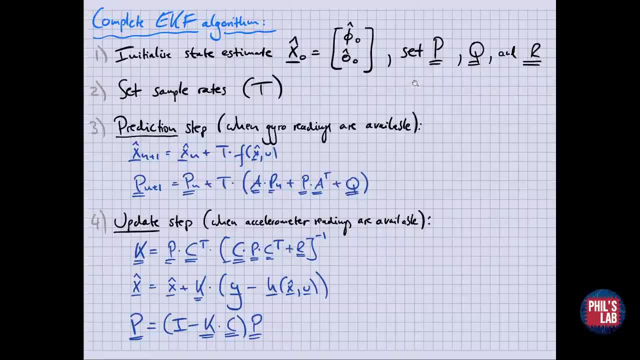 our error covariance matrix p and choose values for the elements of our noise covariance matrix. We also need to set our sampling rate, or rates. Then, whenever we receive gyroscope data, we perform the prediction step, and whenever we receive accelerometer data, we perform the update step. 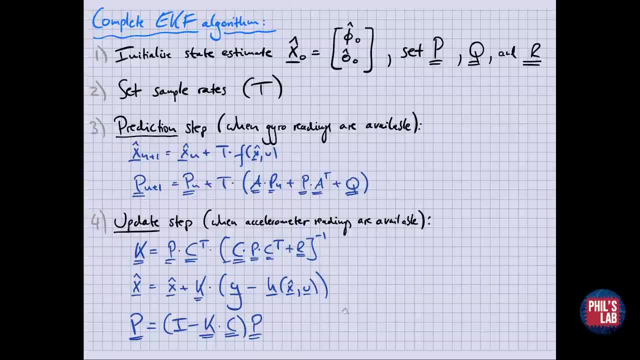 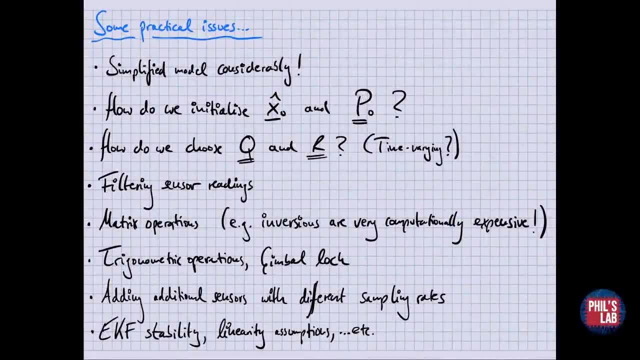 However, when we come to the implementation stage in the next video, there are many practical issues. Here are some examples. We have simplified our model considerably. If we knew more about the physical system- the implementation is running on- we could reduce the error. covariance matrix. 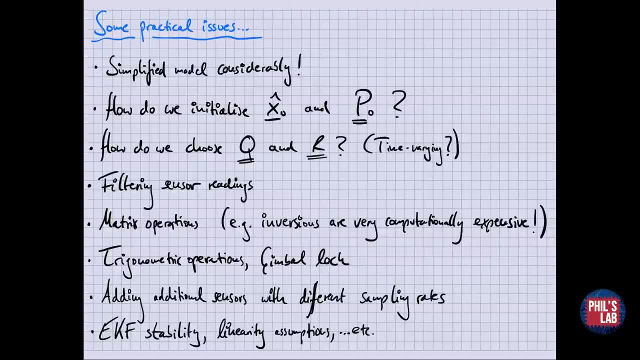 We also need to ask how we can efficiently initialize our state estimates and our covariance matrices. Maybe also q and r could be time varying. We do also need to filter our raw sensor readings before feeding them into the EKF. The question is, how do we? 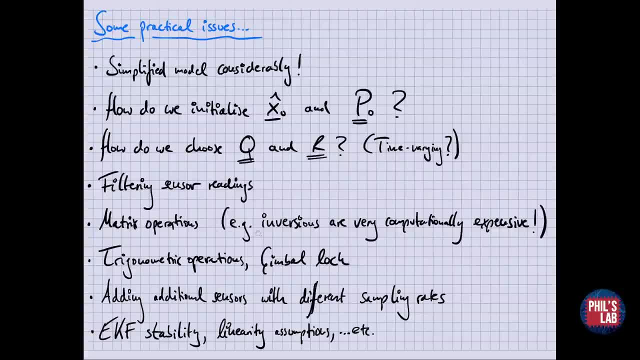 choose these filters. Furthermore, matrix operations are pretty costly, especially as the system dimensions increase. How can we efficiently implement this on a microcontroller? Trigonometric operations are also quite costly, and in addition the use of Euler angles can lead to a phenomenon known as gimbal lock. but more on that again in the next video. We may wish to include additional. 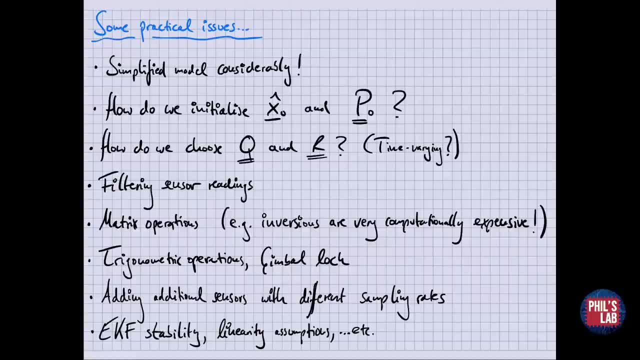 sensors giving us different information at different sampling rates, and how can we actually then implement that? A very important point is also that the EKF can become unstable or that we have wrongly assumed the linearity of the system, and so forth. In the next video we will look at 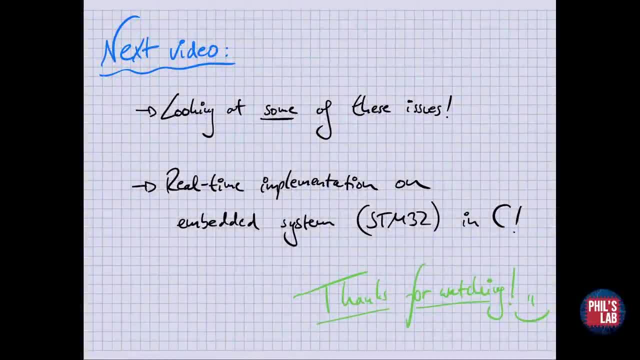 some of these practical considerations. But, even more interestingly, we will look at a real-time implementation of this extended Kalman filter on a real-world embedded system using C. Thanks for watching and I hope to see you again in the next video. If you've liked the video, please give it a thumbs up and please do subscribe to the. 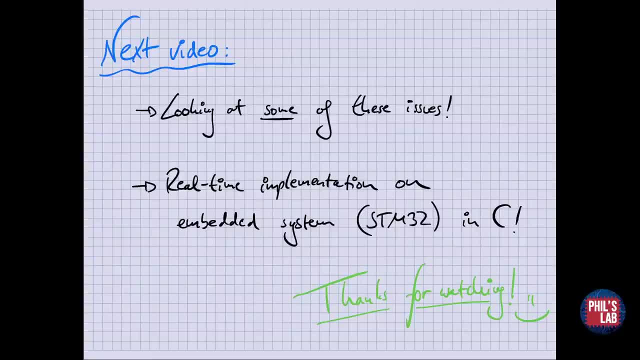 channel for more content on signal processing electronics and PCB design. Thank you.